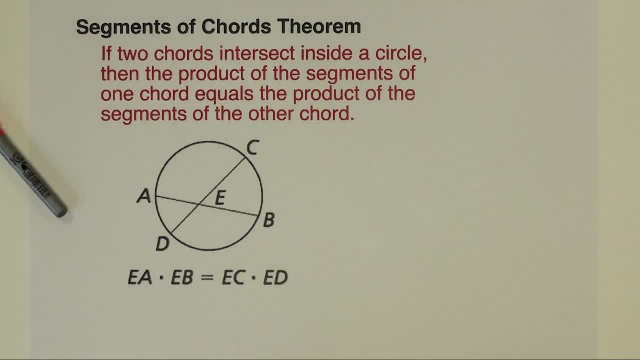 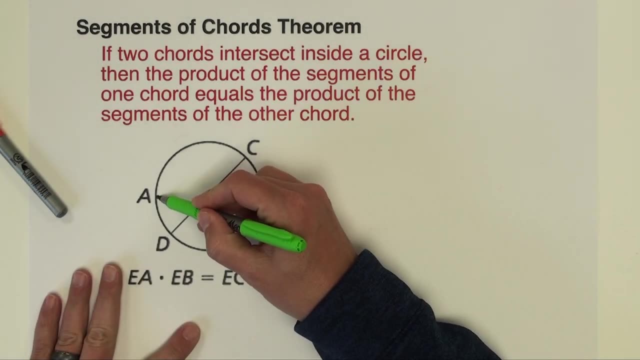 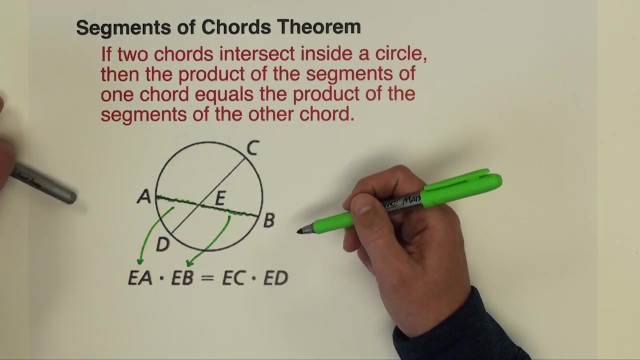 the product of the segments, of the other chord. So let's find those pieces in the diagram here just to kind of color code them, to kind of highlight what we're looking at. We've got these two pieces, two segments, on segment AB. So we've got EA, times, EB, and the product of those two segments is going to be equal. 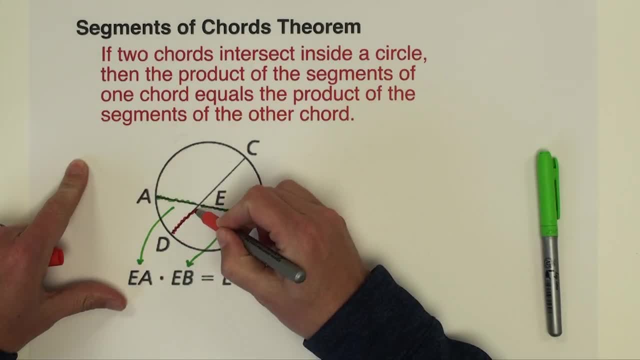 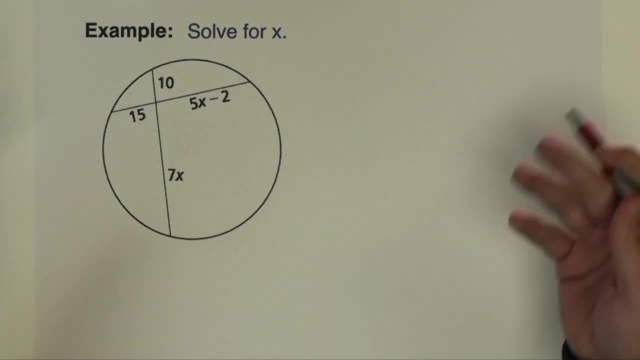 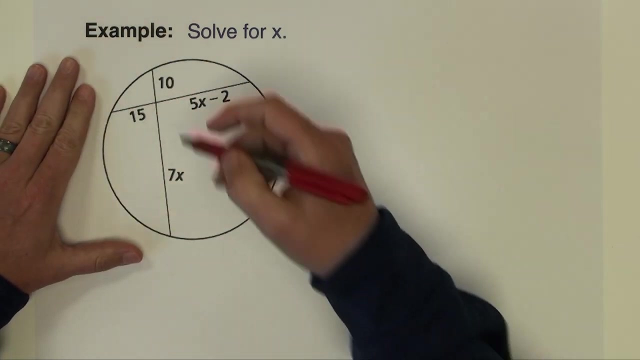 to the product of the two segments of the other chord. So you see those pieces here. Alright, let's see that first theorem, this first theorem, in an example problem. Directions in this first problem are simply to solve for x. We see this again, familiar setup. We've got a couple of chords intersecting inside the circle. 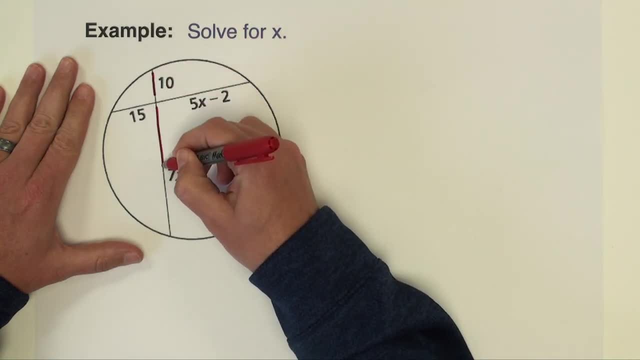 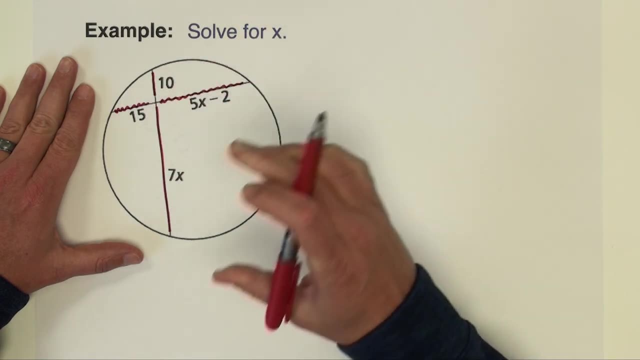 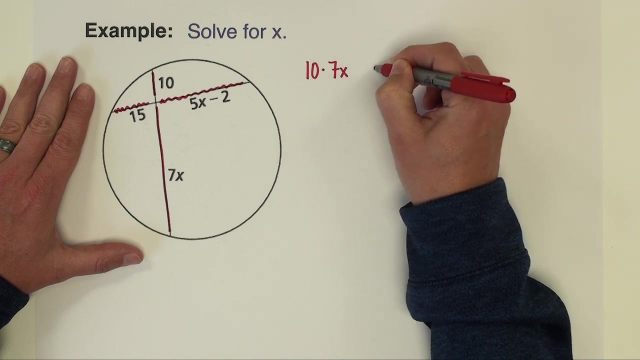 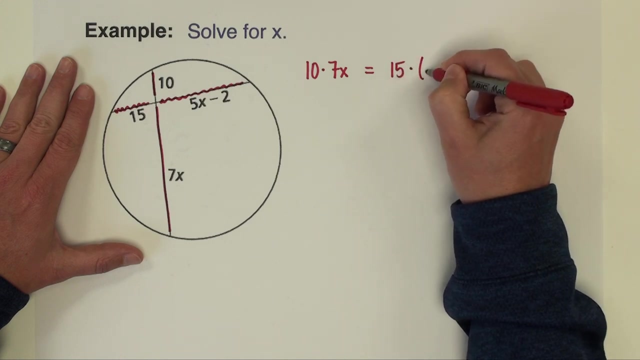 I've got these two segment pieces on one chord and then these two segment pieces on the other chord. So what we're going to do is find the product along each chord. So I'm going to take 10 times 7x and that's this chord. I'm going to equal that to 15 times 5x minus 2.. Alright, 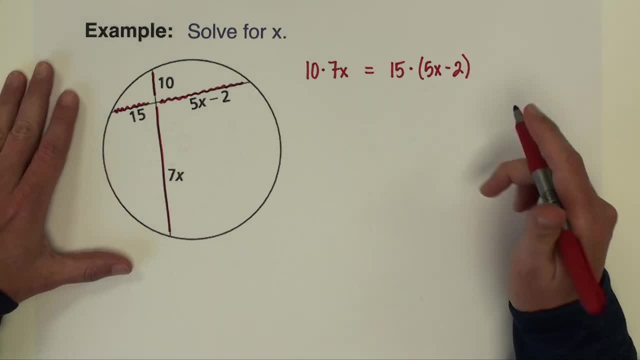 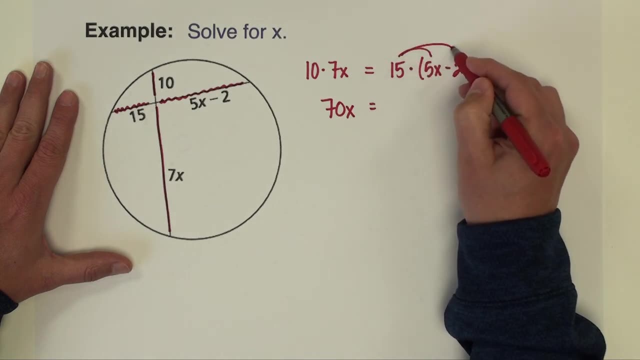 so there's our setup. If we go off of that theorem, now we just need to solve this equation: 10 times 7, 70x equals We'll distribute the 15.. So 15 times 5 is 75x, and then we'll have minus: 15 times 2 is 30. I'm going to take 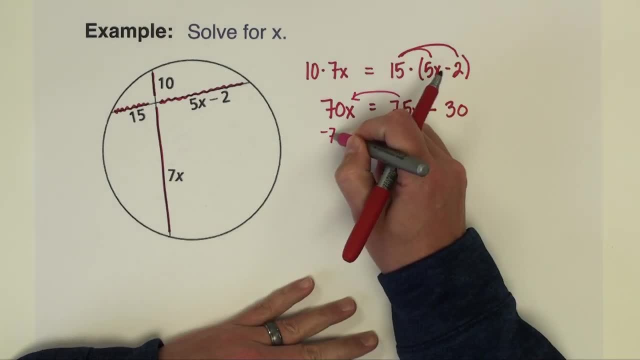 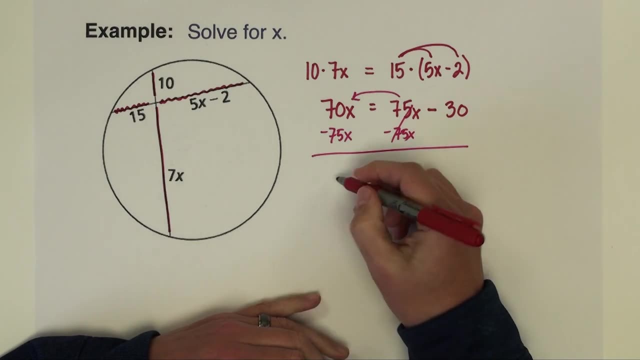 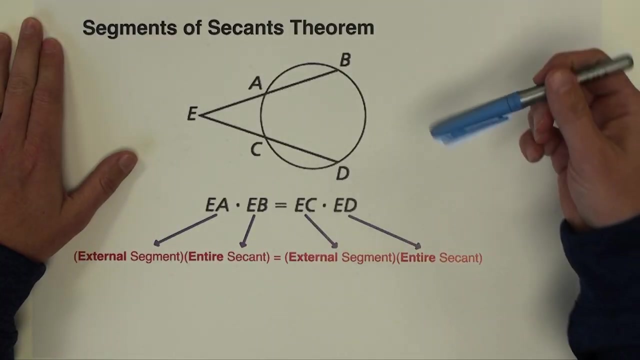 the 75x and subtract it over to this side. So I've got negative 5x equals negative 30 and if I divide by negative 5, we get x equals 6.. This next theorem is called Segments of Secants theorem. Instead of just presenting you with 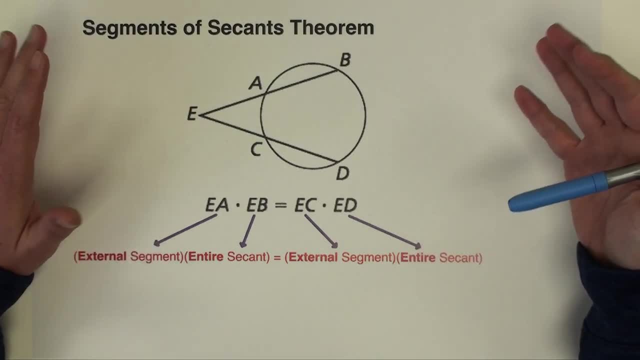 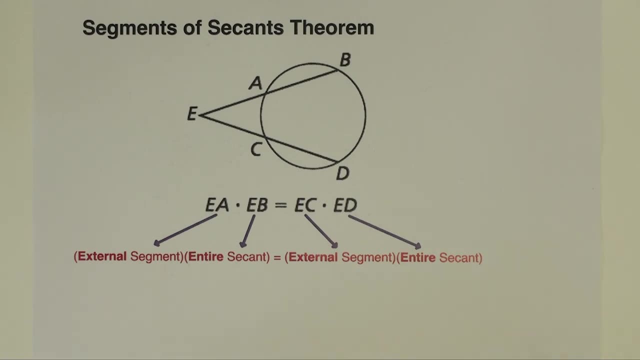 a wall of text. that is the theorem. I thought we'd just look at a picture. I've got a formula here and kind of a description of the formula. Well, let's kind of find the pieces in this diagram as it relates to this equation down here. 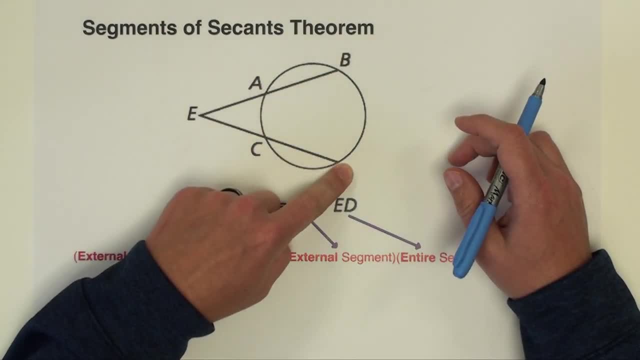 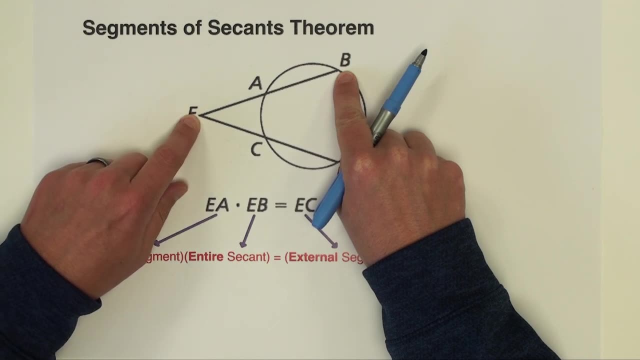 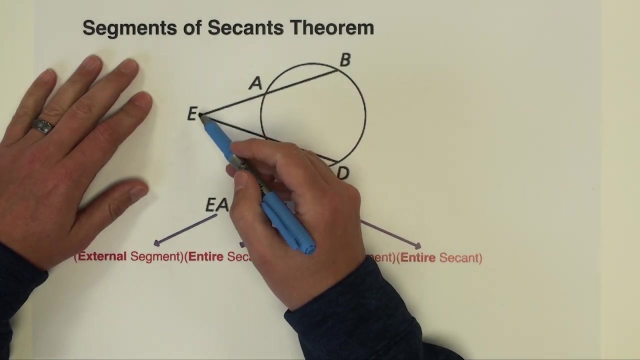 So the way this works, we've got two secant segments, あの and or segment itself. EB is divided into a couple smaller pieces here, And so here's how this is going to work. You start with the external segment, So I'm going to start with EA right here. 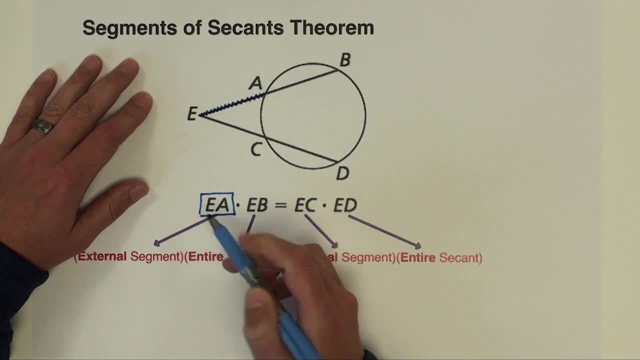 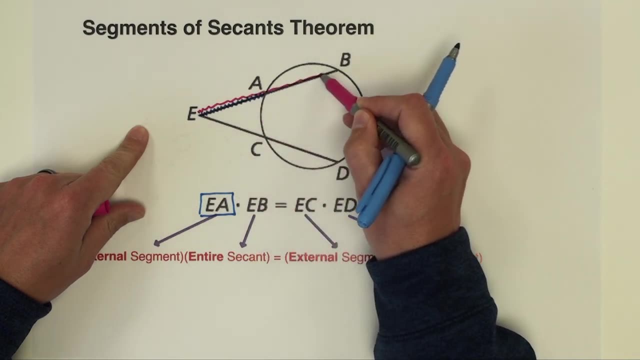 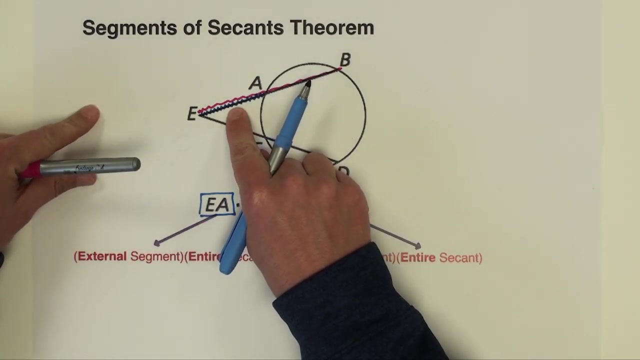 And we see that right here. And I'm going to multiply that by the length of the entire segment EB. see that right here. Okay, so it is the, the outside or external piece. we're going to multiply by the whole thing, And that's one side. we're going to do the exact same. 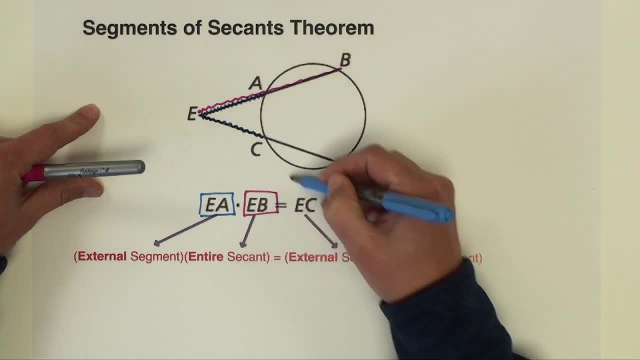 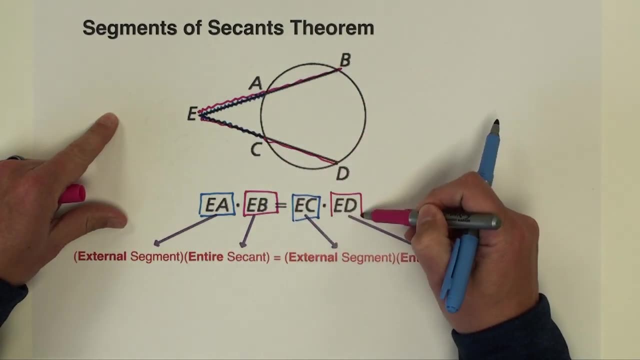 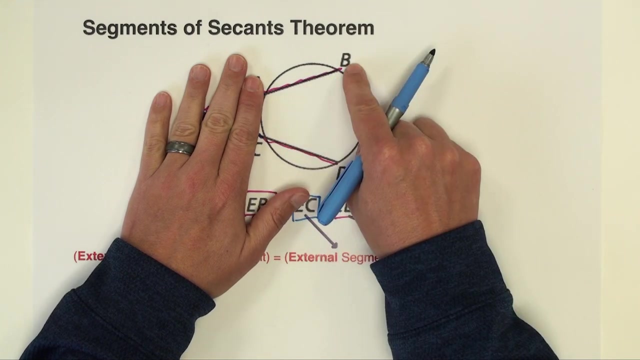 thing to the other secant, we're going to take the external part And then we're going to multiply. that times the whole thing, Okay, so? so that's how the equation works. We never use just the interior piece. Okay, it's not going to be used, It's it's outside. times all of it equal to the. 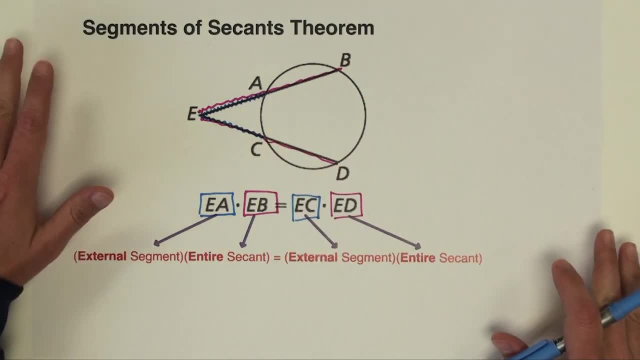 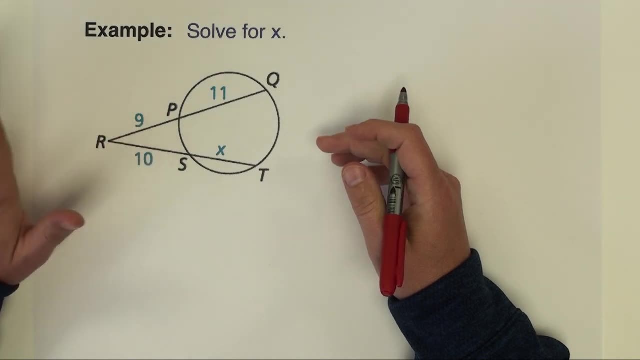 outside times. all of it, All right. let's see that in an example problem. All right, here we go. Another problem where we're asked to find the value of x: here we've got these two secant segments. So I begin this by, and it doesn't matter which segment you take, But I'm going to begin. 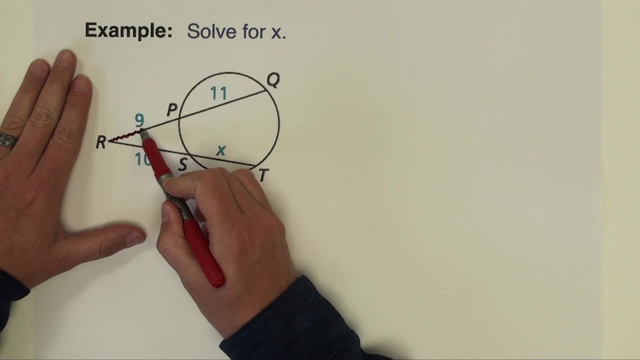 this on the top segment, I'm going to take the outside piece, which has a length of nine, And I'm going to multiply it by the length of the entire piece. Now that's confusing. Sometimes we want to take nine times 11. And that's not going to be correct because the entire 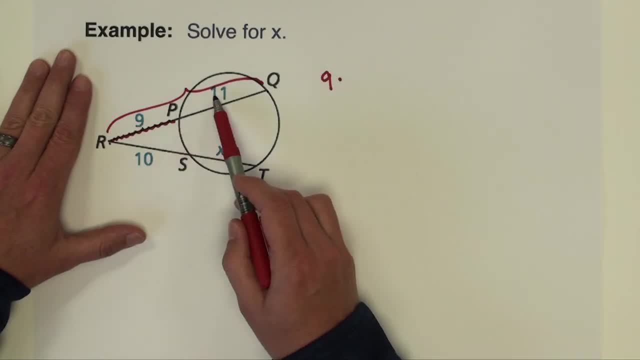 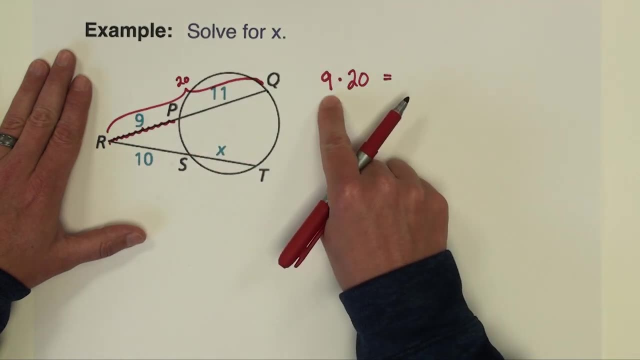 piece does not measure 11.. If you add these pieces together, nine and 11 makes the entire length 20.. And that's what we're going to multiply by. So the outside piece times the entire thing, and we do the same thing on the other. 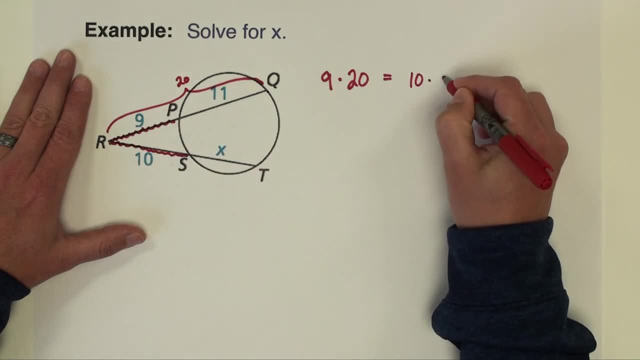 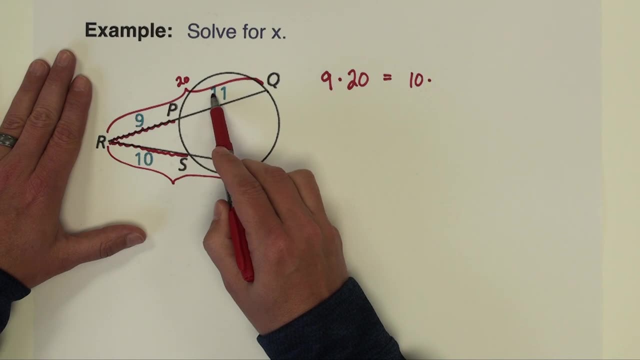 secant. I want the outside length, which is 10, I'm going to multiply by the length of the entire thing, And the entire thing, just like up here, nine plus 11 gave 20, I'm going to do 10. 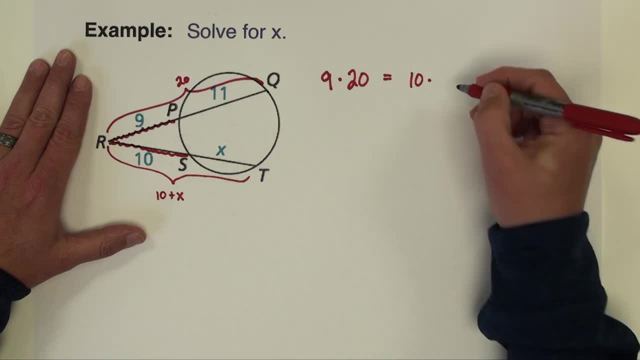 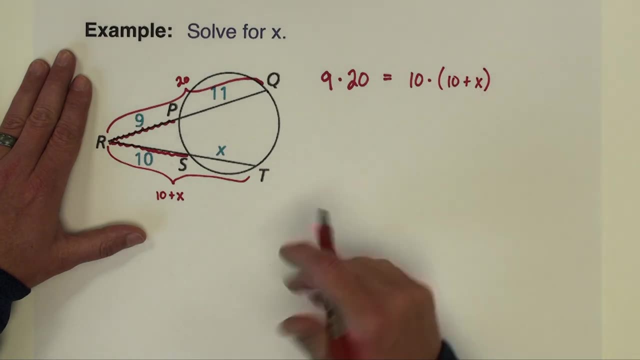 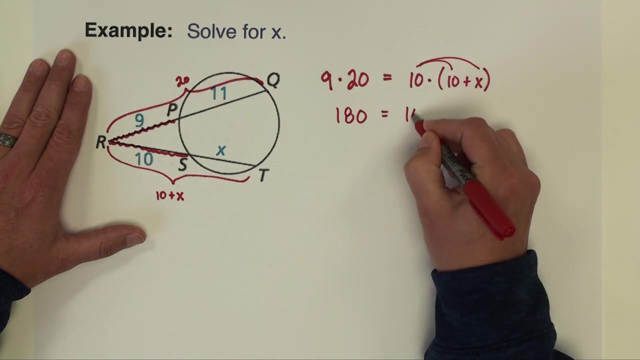 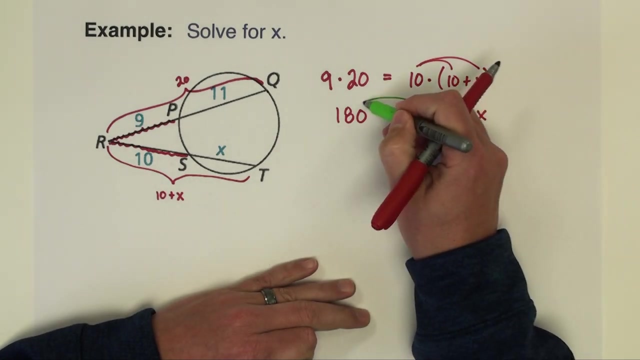 plus x. only. I can't put those together any more than that. So there's the beginning. Now we can start to solve this equation. nine times 20 is 180 equals, and we'll distribute the 10. there we have 100 plus 10 x. And take our 100 and subtract it to the left hand. 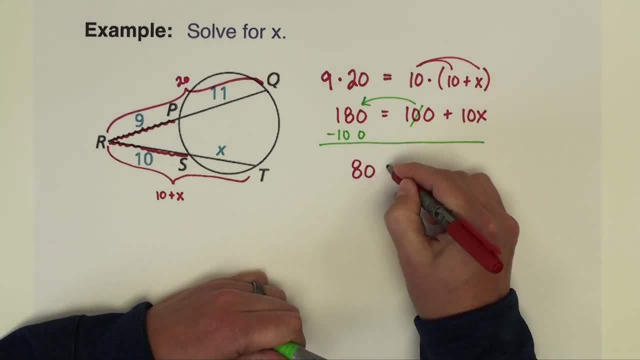 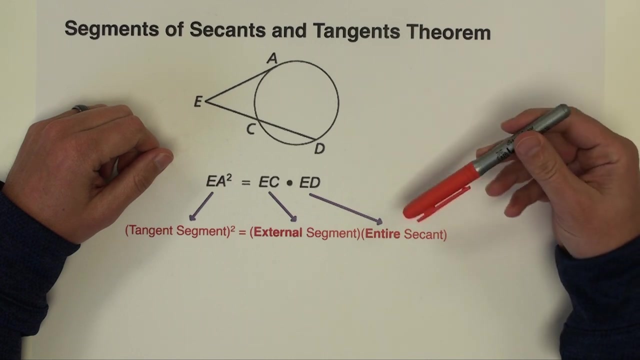 side, giving us 80 equals 10 x, and divide both sides by 10, we get x equals eight. All right, we're going to close this video with one more thing. So let's look at the secant theorem And then one more example problem to support this theorem. 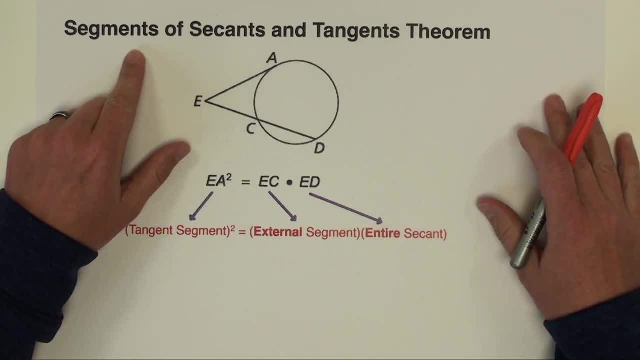 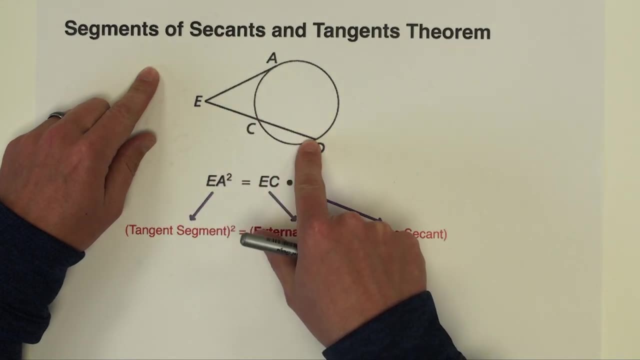 This one is segments of secants and tangents theorem. So here we've got another secant line, like we had in the last theorem and example, But this time we also have a tangent segment, And so how we deal with that is very similar, but it looks a little, maybe a little bit different down here. 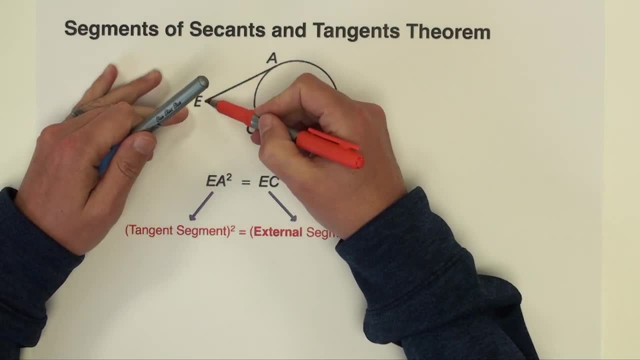 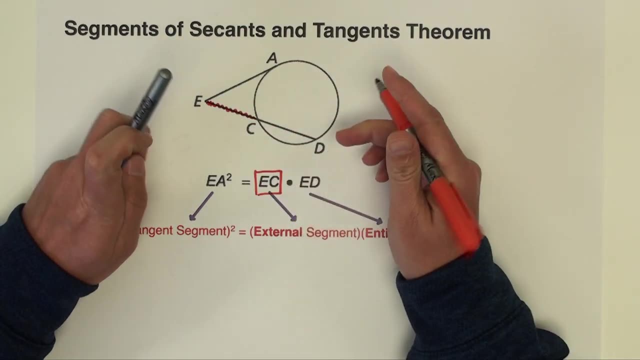 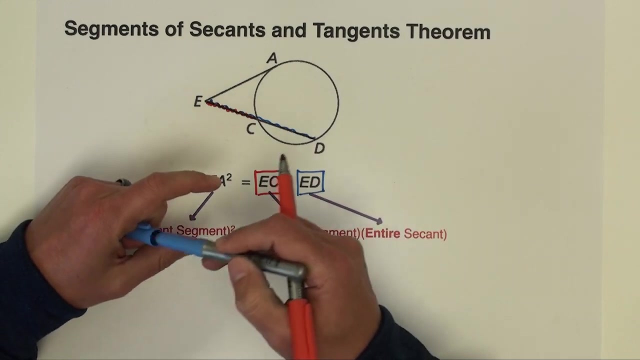 First, let me look at just the secant segments. So look at, let's look at the bottom first. we've got the, got this outer piece, ec. we're doing that again and then we're going to use the whole thing ed. okay, so there's no difference at all to how we do that from the previous theorem, it's the. 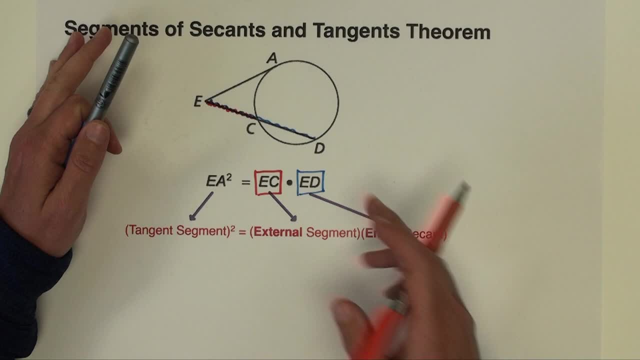 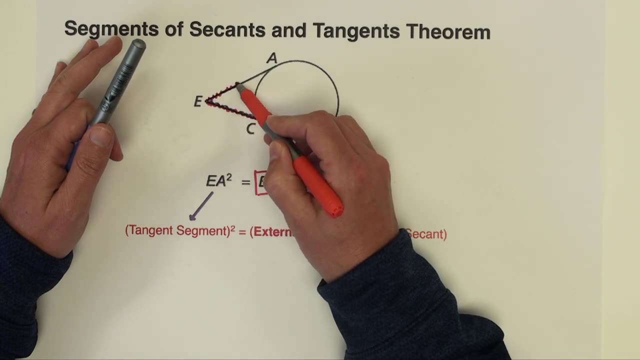 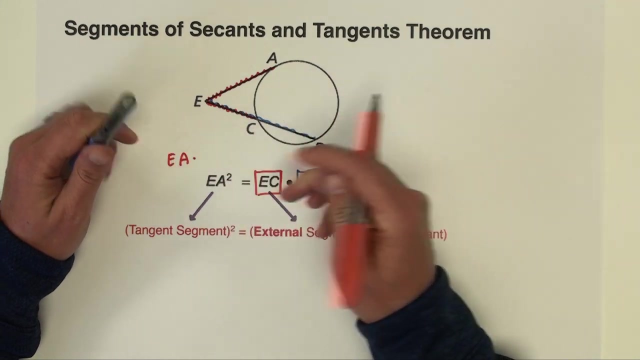 external piece times the entire segment. now, when we go to the tangent segment, we're actually going to do the same thing. we're going to take the external part, which is ea. let me write that out. i'm going to take the external part, ea, and then we're going to multiply that by 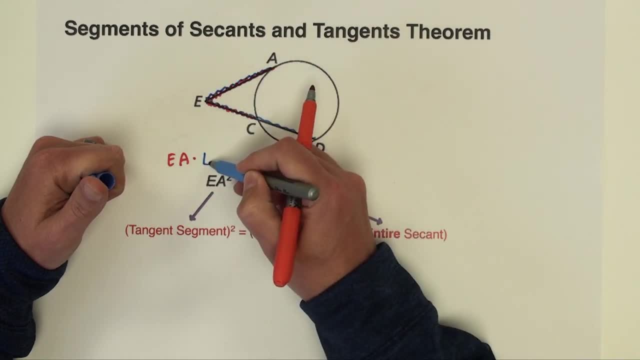 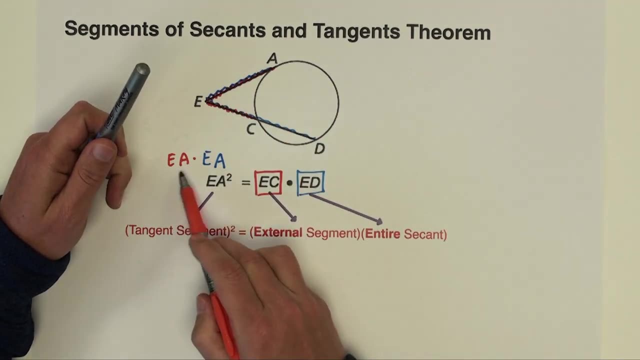 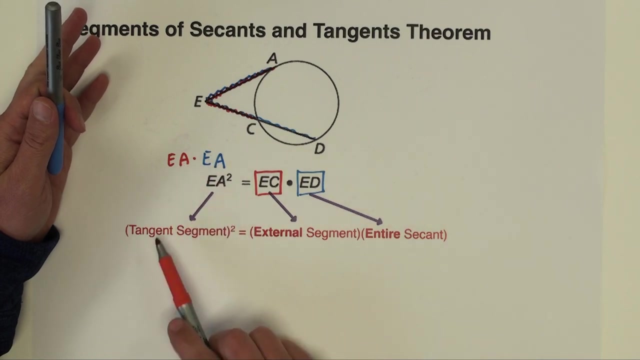 the length of the entire thing, which just so happens to be ea again. so the formula you can see it's written a little bit differently. it's just written as ea squared, as that would be a way to re-express ea times, ea. so taking the tangent segment, squared times, and then on the secant, the external times.